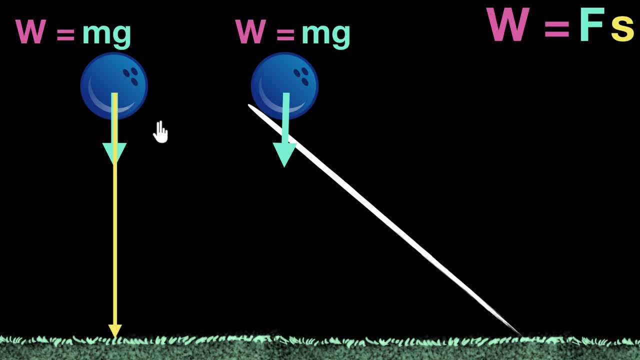 So the displacement is just the height of the ball, And so in the first case the work done becomes mg times h. But what about the second case Now? in the second case, the displacement is from here to here, which is more than the height of the ball right. 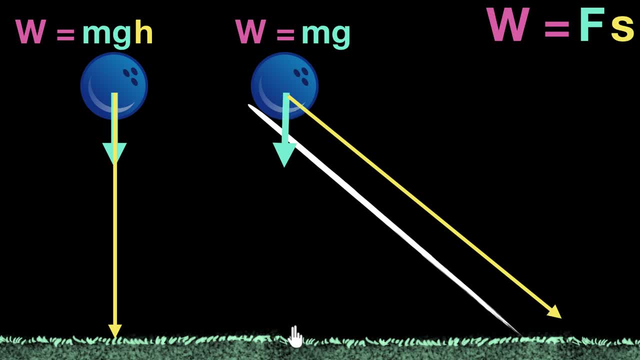 This length, as you can see, is larger than this length, larger than the height, And so if we call this as let's say s, we might say in this case the work done will be mg into this displacement And therefore we might conclude that more work. 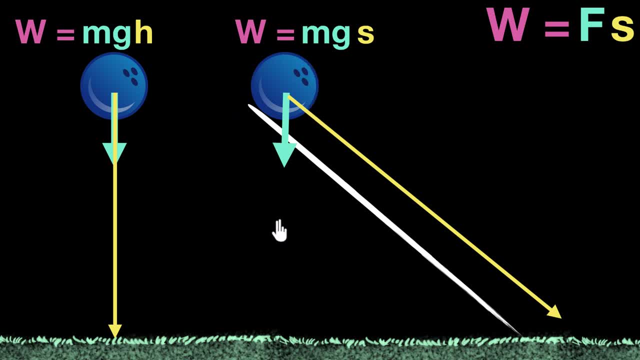 is done by gravity in this case, right? Well, one important thing to see over here is that the force and the displacement in this case are not in the same direction. You see, they're in a different direction, And whenever we say, we're calculating work. 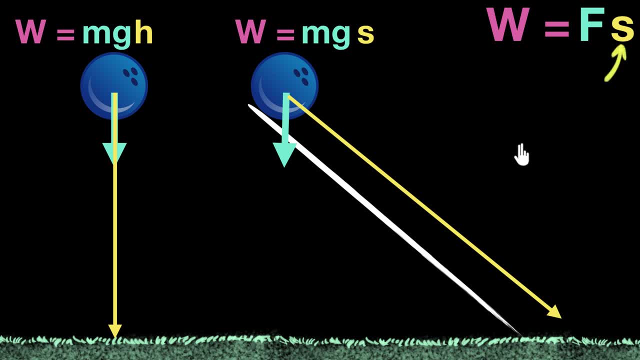 as force into displacement, that displacement has to be calculated in the direction of the force, And so I guess the goal of the video is to try and figure out, whenever the force and displacement are not in the same direction, how do we calculate work done. 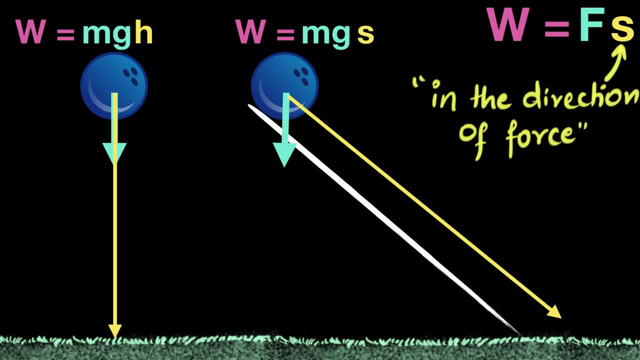 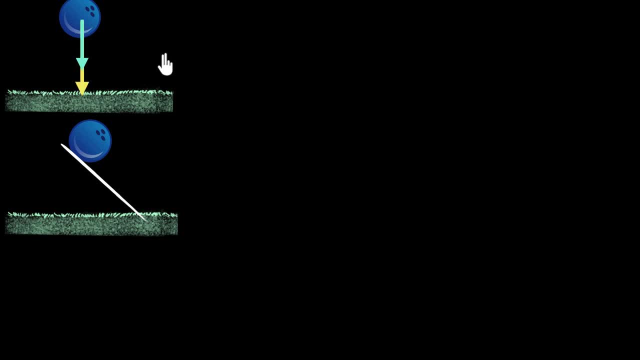 What is the meaning of this statement? So let's look at these two cases in a little bit more detail. okay, So in the first case, the force of gravity is down and the object just falls down, No surprise. In the second case, gravity is down. 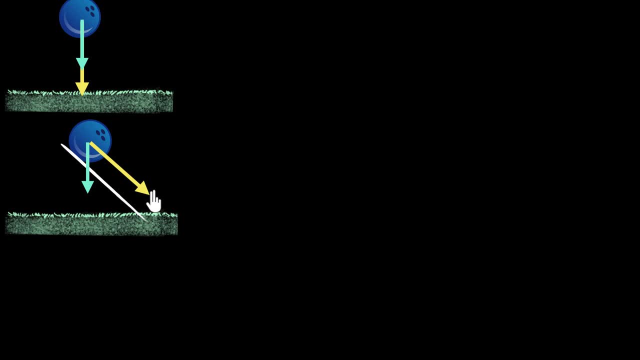 but the ball is falling down at an angle. It's sliding down at an angle, So again, not surprising. but what does it mean? This means gravity can make things accelerate in other directions as well, not just down, but in other directions as well. right? 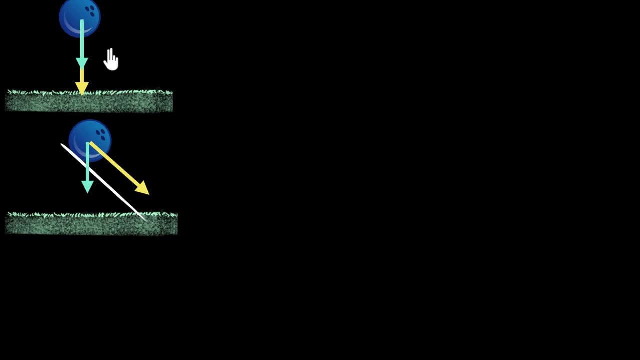 But there's a difference between these two. In which case do you think the ball accelerates more quickly? Well, I'm pretty sure you agree. it's in the first case. In the first case, the ball actually as it is. 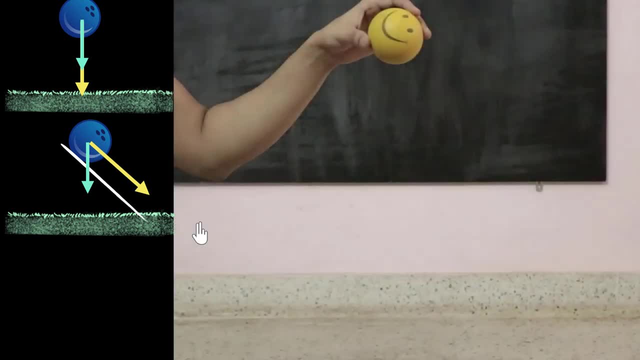 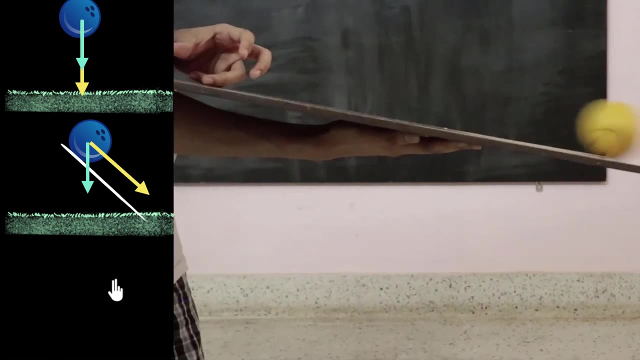 it very quickly compared to the second one Here. let me show you this. So if I drop the ball, see how quickly it just fell down. The second case I'll make it slide and now notice it's a little slower than before. 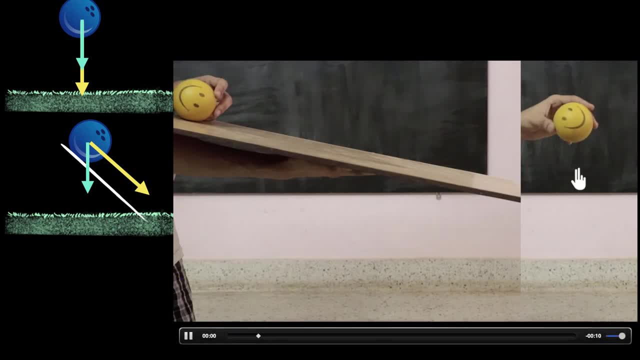 Again to see it clearly, let's do a comparison side by side in slow motion and you can see immediately the ball here accelerates down, but over here, notice it's so much slower. So the ball accelerates much slower here compared to this. 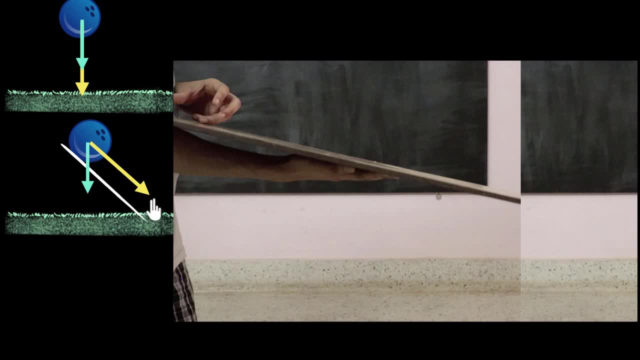 So what can we conclude from this? Because the acceleration is slower, we could say the effect of gravity felt by this ball must be less right, Because it's feeling less force and therefore smaller acceleration. So we can conclude that gravity has an effect. 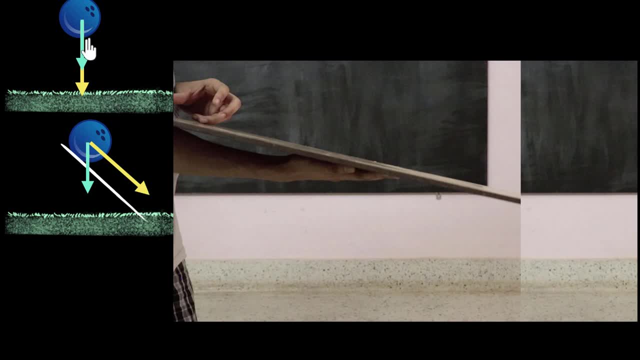 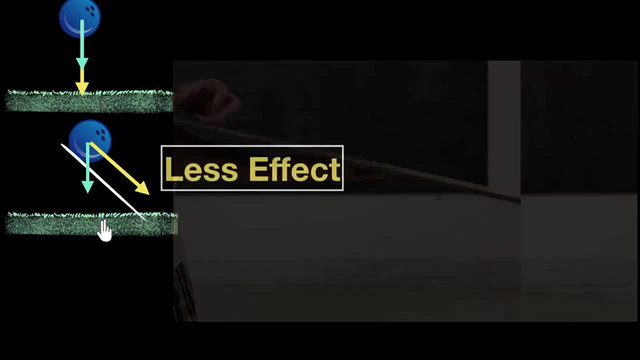 in this direction, but that effect is smaller compared to the previous one right. So at an angle the effect of gravity reduces. So we could say: less effect along this angle. Okay, in the third case, what we'll do is: 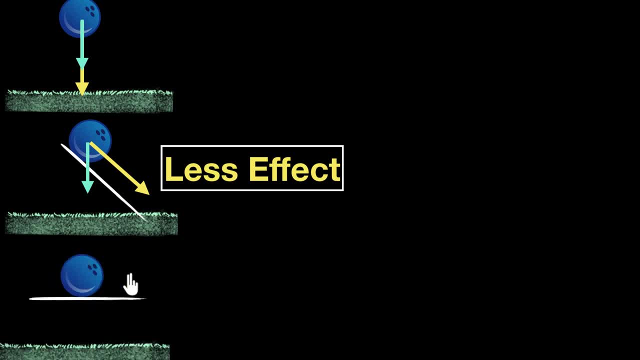 we'll try to make that object slide horizontally due to gravity. What'll happen? Well, gravity's acting down and we're trying to make this object go forward. let's say: Do you think this is gonna happen? I'm pretty sure you agree. 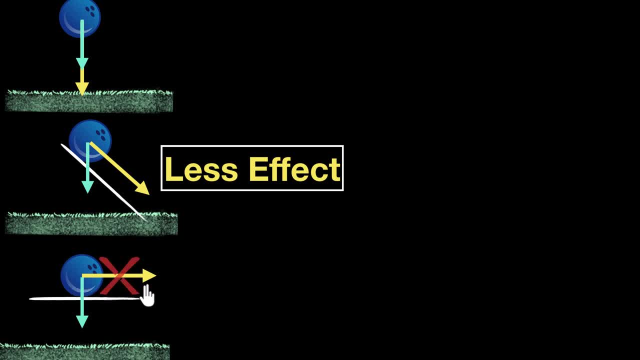 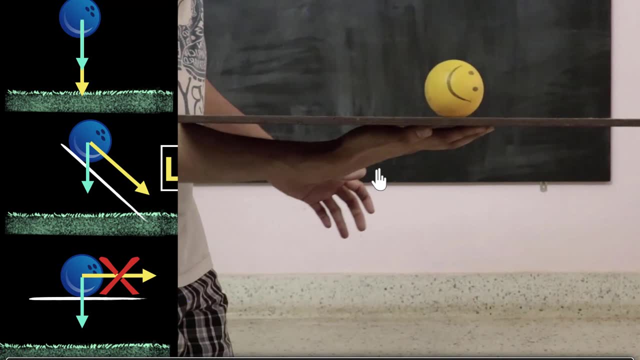 nothing's gonna happen in this case, right? This object is not going to move at all. Again, I can just show you that I'll just keep an object. This time it's horizontal. Yeah, the ball is moving because my hand is shaking. 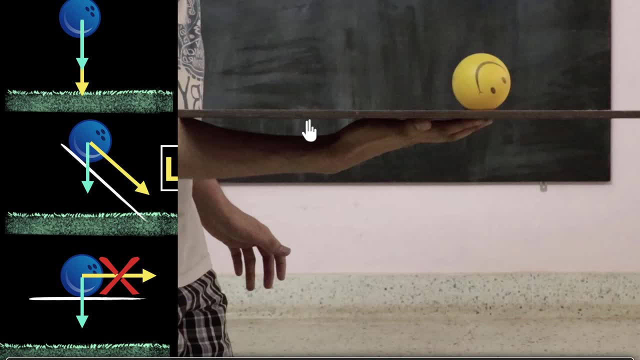 but I'm pretty sure you agree that the ball is just gonna be at rest, if this was perfectly leveled right. So in this case gravity cannot affect the motion at all. So we can say that gravity has no effect in the horizontal direction. 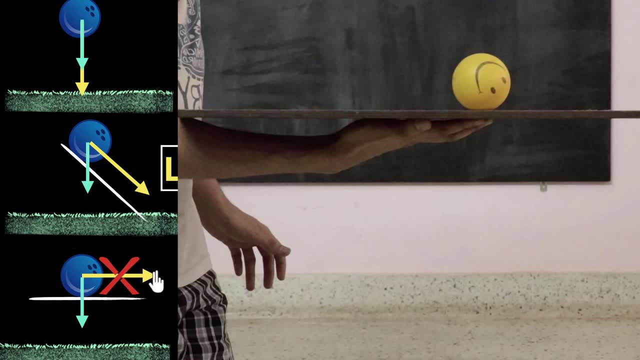 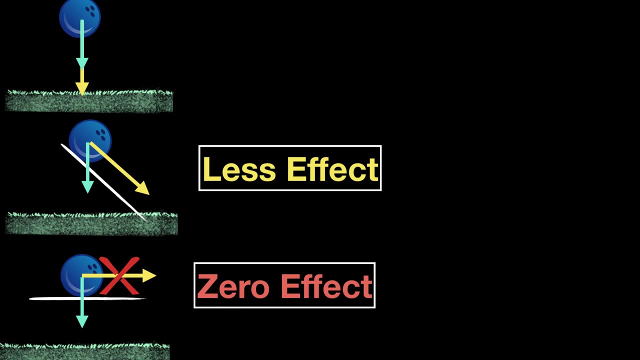 Does that make sense? Because it's unable to accelerate this ball. So in this case, we can say: gravity has zero effect. Now, before we put all of this together and try to make sense of this, let me tell you that this is not just for gravity. 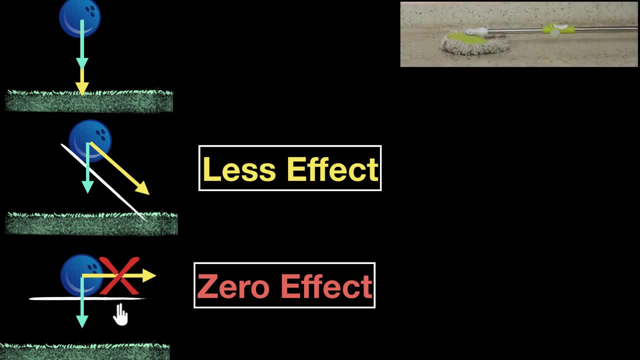 This can be seen in any force. To give you an example, let's say you take a mop and you push it forward. Then you'll expect the mop to accelerate forward. It'll speed up in the forward direction. No surprise, right? 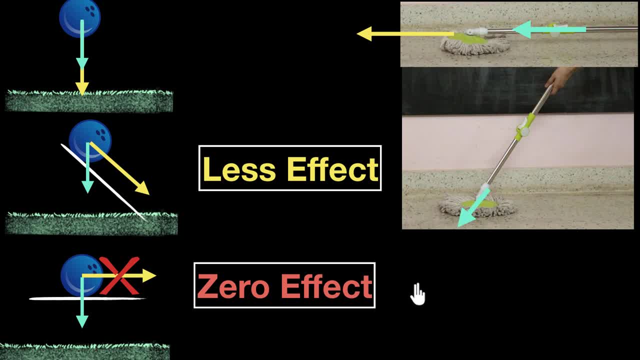 But take that mop and now push it at an angle, And again that force can accelerate it. Meaning notice, even though this force is acting at an angle, it has an effect in this direction, Just like what we saw over here. 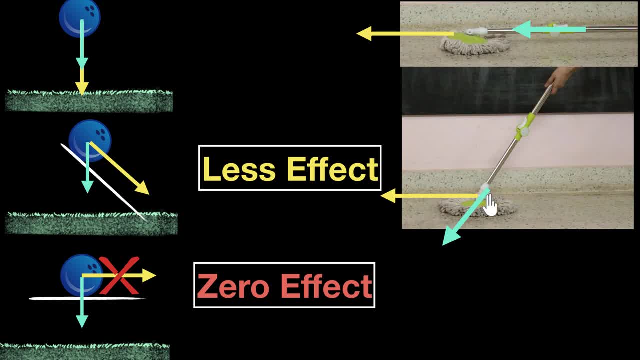 So this force also has effects in other direction. But again, you might agree that over here the effect is a little smaller, because now the mop will not accelerate as much as it accelerated in this case, right, So the effect has reduced. 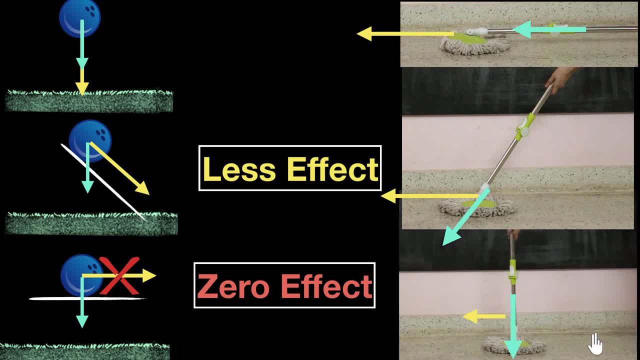 And eventually, if you push the mop straight down now, you'll see it has absolutely no effect in the horizontal direction. So this force has zero effect in this direction. So if you put it all together, what do we understand? First of all, we see that forces can have effects. 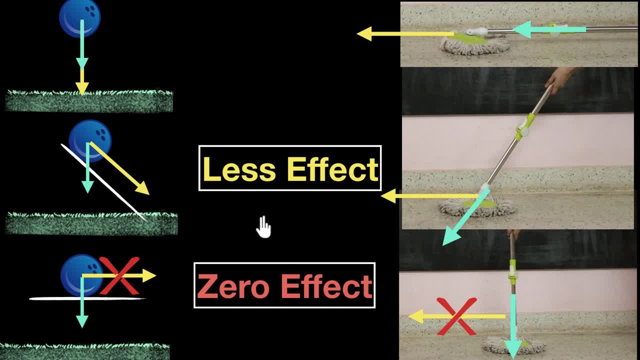 in other direction as well. But what's important is that as the angle between the force and the motion increases, as this angle starts increasing, the effect starts reducing. You see, the effect is maximum when the force and the motion are in line with each other. 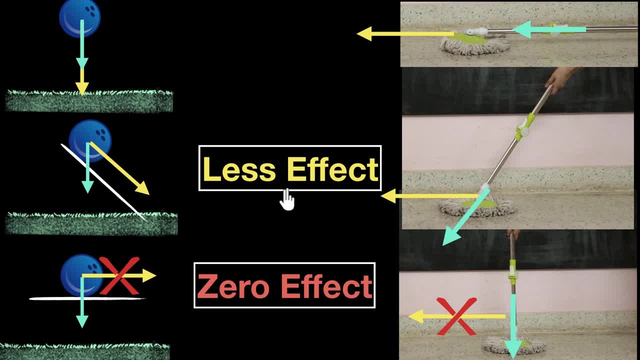 But as the motion starts making an angle with the force, the effect reduces, And when the angle becomes 90 degrees, as you can see, the effect becomes zero. This is the most important thing. okay, This means that forces have no effect. 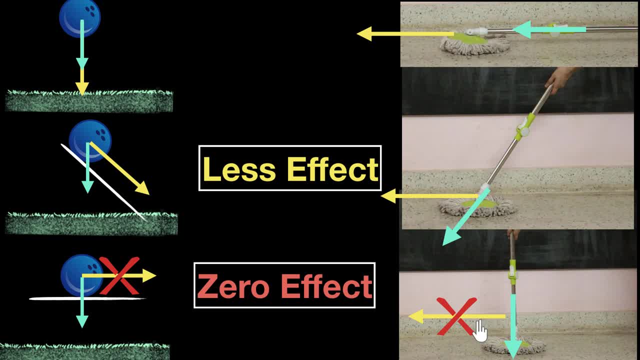 in perpendicular direction. It has zero effects in perpendicular direction. So what can we say about the work done in this particular case? Well, let's take an example. So imagine I take a ball and I keep it on a perfectly horizontal slide. 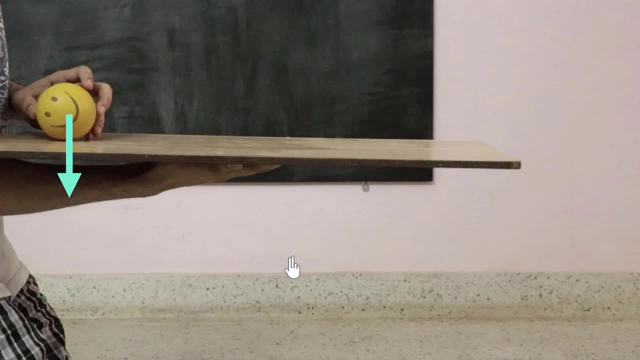 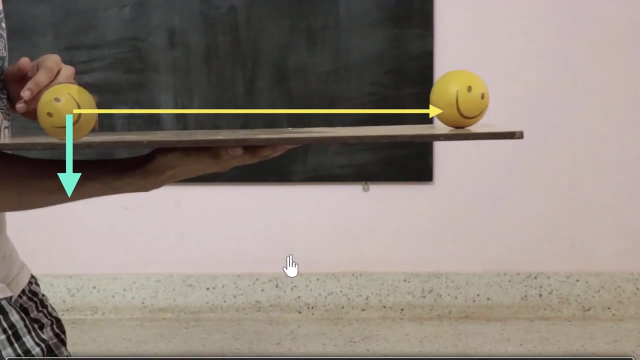 And let's think about the work done by gravity. Gravity is pulling it down. Let's say, I push this ball now And make it displace horizontally. What is the work done by gravity? Can we just say it is the gravitational force multiplied by the displacement. 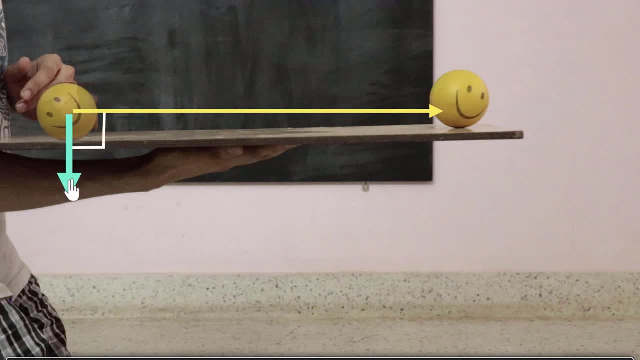 No, Because the angle between the gravity and the displacement is 90 degrees. we can now say: gravity has no effect in this direction, like we saw earlier. So gravity is not causing this displacement at all And therefore we can say: the work done by gravity is zero. 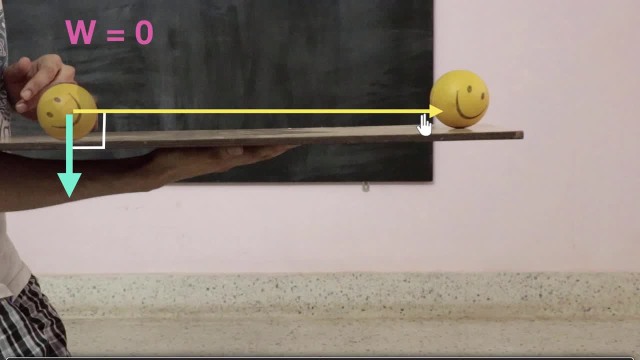 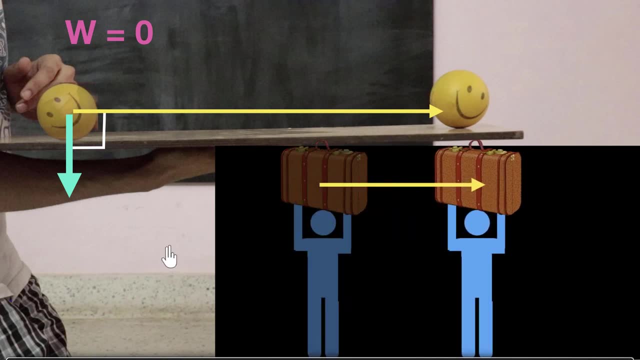 Because gravity is not the one that displaced this body. Does that make sense? So, in a similar manner, imagine somebody is carrying a luggage on their head And let's say they move forward displacing that luggage. What is the work done by their force on the luggage? 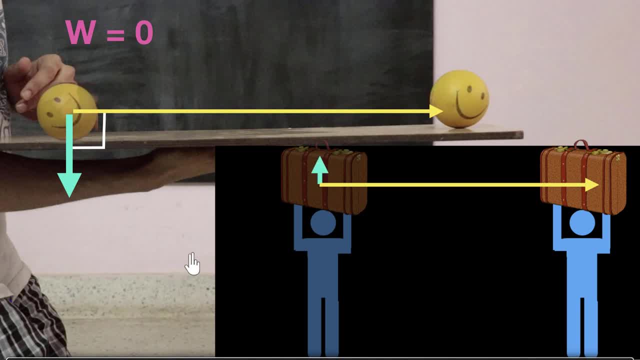 Again, that's zero. Why? Because they are pushing on the luggage up and which is perpendicular to the direction of the displacement, And so we can say: this force has no effect in this direction, It did not cause this displacement at all. 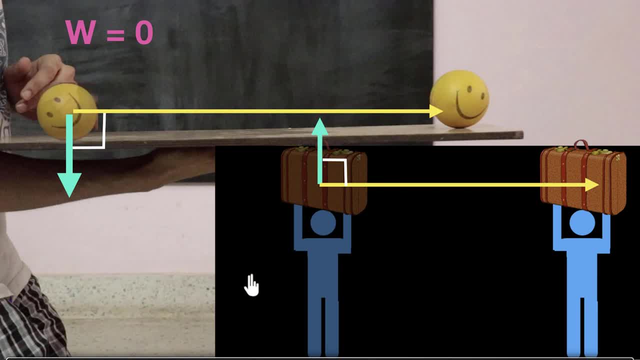 And therefore the work done by this force on the luggage must be zero. And so in general, if the force and displacement are perpendicular to each other, work done by that force must be zero. So now let's see how this knowledge helps us. 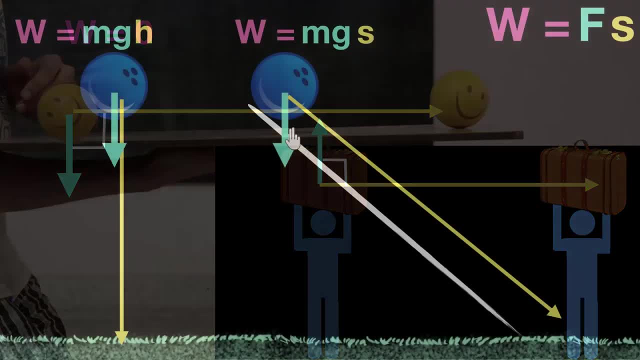 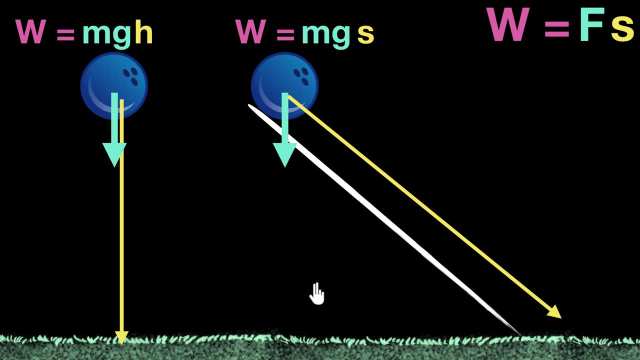 in answering our original question. So we want to calculate the work done. in this case, right Now, instead of the ball sliding straight down, let's assume. let's assume for a moment that the ball is going on a staircase, So let's assume that the ball is going forward. 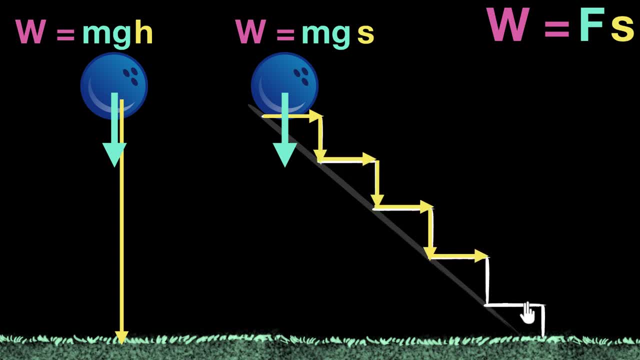 then coming down, then going forward, then coming down, and so on and so forth. Let's assume it's going that way. I know it's not really doing that, but let's calculate the work in this case first. It'll help us to figure out what happens in the work. 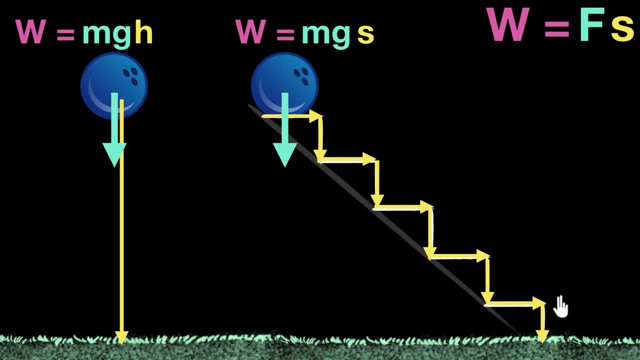 in the sliding case as well. So what is the work done in this entire motion? Well, again it's going to be force times, displacement. We know the force, which is mg, but what is the displacement? Should we take this entire displacement? 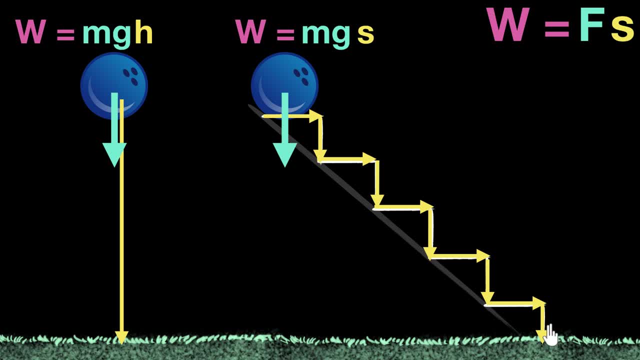 Should we add up all the displacement? Should we add up all these displacements? No, because we know now that during the horizontal motion, gravity is not doing any work, So this displacement doesn't come into the picture. During the vertical motion, gravity is doing work. 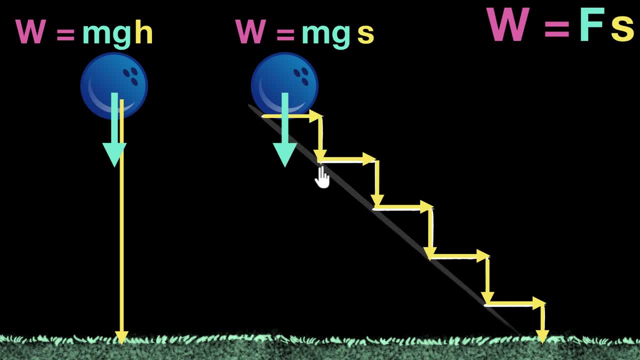 Gravity is pulling and making it displace. So this matters Again during the horizontal motion. that displacement doesn't matter Again during the vertical motion, it matters. So during the horizontal motion, since the work done is zero, we can just get rid of the displacement. 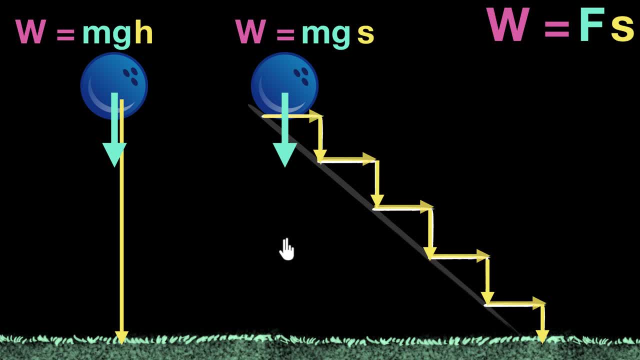 That displacement doesn't come into our formula, So let's get rid of that displacement. And so the only displacement that matters to us is the one that happens in the direction of the force of gravity. right, And that's what we meant earlier. 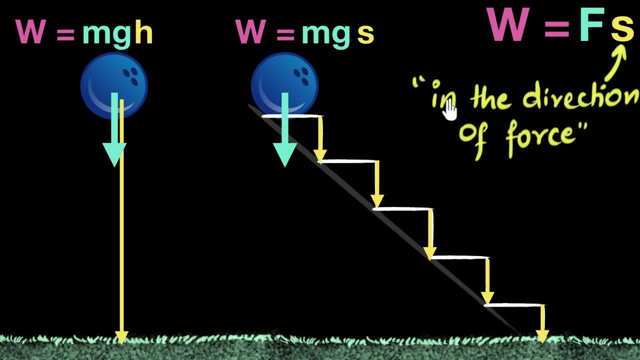 that when you're calculating the work done, what matters is the displacement that happens in the direction of the force. Only that displacement should come into the picture. Okay, so what is this total displacement? Well, we just have to add all of them up. 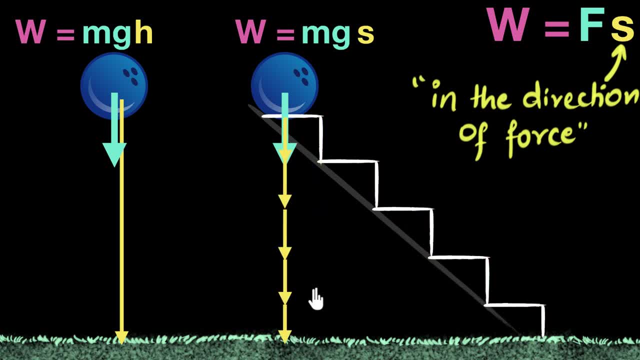 Now, if we add all of them up, notice what we get. We just get the entire height of the ball from the ground, which means that displacement over here has to be Hedge itself. Therefore, the work done in this case is exactly the same as the work done in this case. 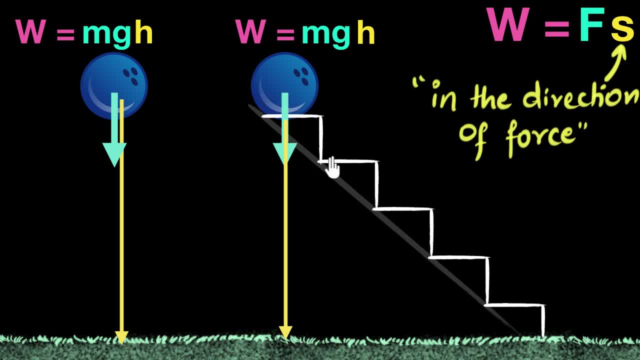 So even though the ball is going down on a staircase, going forward and going down and so on, the work done by gravity must be done, must be the same. Now, of course, you might say, well, okay, but that doesn't answer my question. 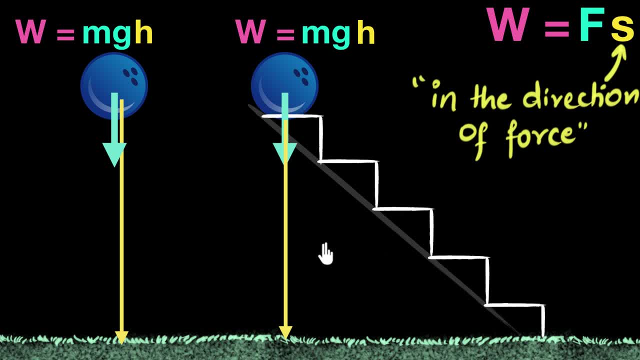 Our original question was not on a staircase. it was going down on a slide right. How do we answer that? Well, we'll come to that Now. instead of thinking of a big staircase, let's assume we made the step size smaller. 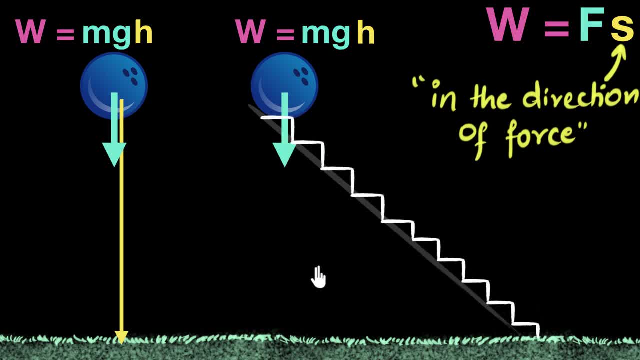 so we had a longer staircase. Okay, now again, imagine the ball goes forward and comes down, and so on and so forth. What would be the work done? Well, again we don't have to worry about the horizontal displacements, because the work done by gravity would be zero, right? 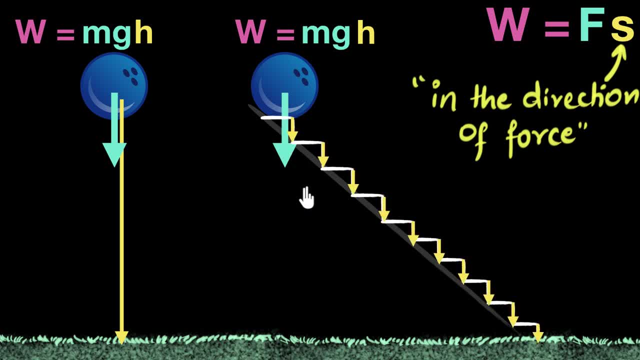 In the perpendicular direction, gravity has no effect. So the only displacement that mattered to us is in the vertical direction, in the direction of the force. Again, if we add up all those displacements, notice we end up with just h. So this means even if I make the staircase smaller, 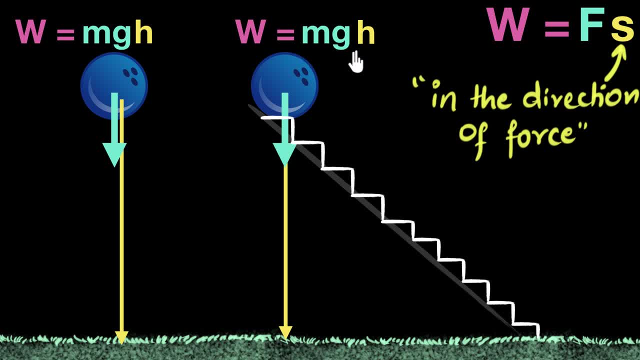 the work done by gravity should still be the same. So now, let me make the staircase even smaller. The work done should still be the same. Let's make the staircase even smaller. The work done will still be the same. Now you can imagine if we go on making the staircase. 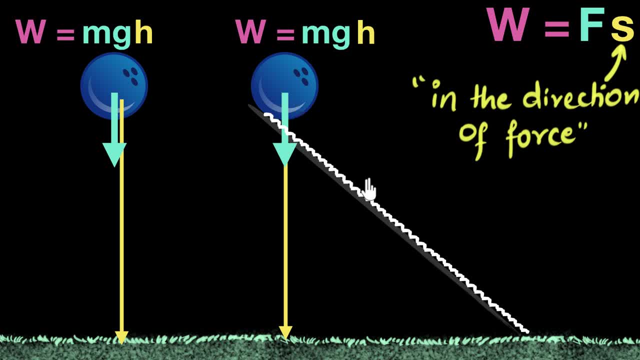 smaller and smaller, and smaller and smaller. the motion of the ball will start becoming smoother and smoother And eventually, if you imagine the staircase, small is super, super, super, super, super small. we can pretty much assume that that staircase is now like the slide. 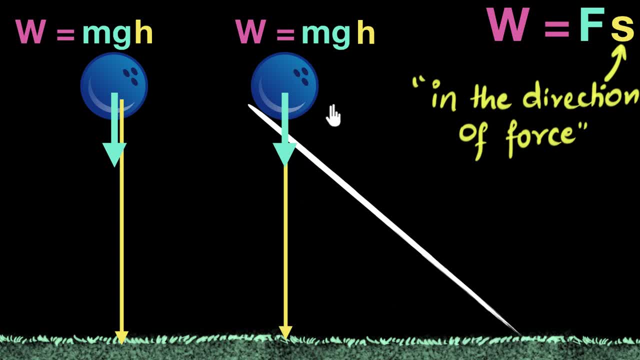 And we can now say that the work done in this slide must also be the same. So in both the cases, gravity does exactly the same work. Amazing, isn't it? Now we can extend this even further Instead of going on a slide. 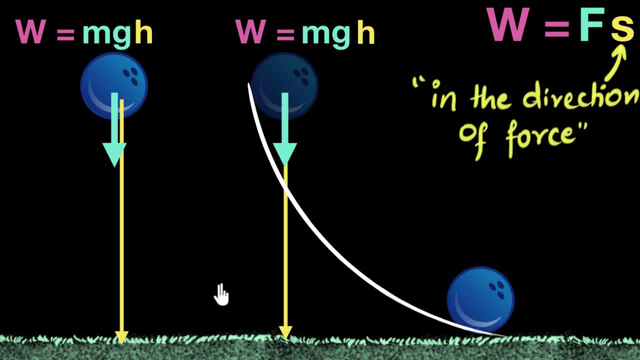 let's say the ball went on some curve like this. What is the work done by gravity in this case? Again, it should be the same. Why? Because again you can think of it as it's going in a very tiny staircase from here to here. 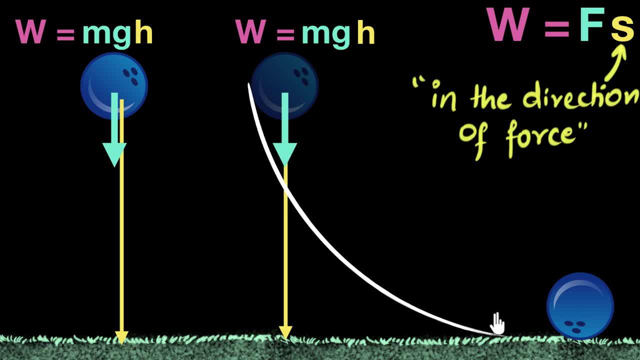 And when you add up all the displacements, only the vertical displacements will matter, And again the total displacement will still be just h. So even in this complicated, curvy example, work done by gravity is still the same, And so now we can extend this in general. 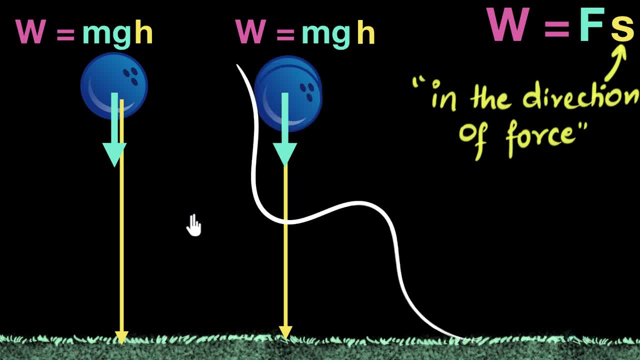 and we can say, even if our ball was going in some crazy weird path, then the work done by gravity will again be just the same. So it seems like the work done by gravity doesn't depend upon what path it takes to go from one point to another. 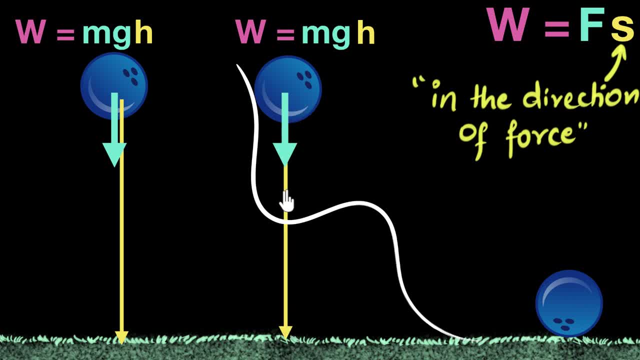 It only depends upon the height that it covers right. The height is all that matters. It does not depend on the path. This is important because tomorrow, if we have our object going in some crazy path and we are asked to calculate the work done by gravity, 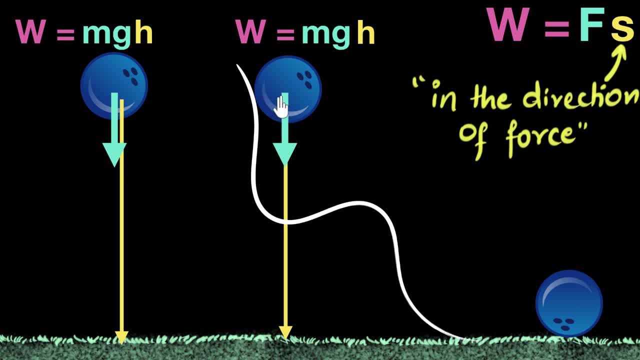 we don't have to worry too much about the path taken. We just say it's the force into the height that it covers from one point to another. And so what did we learn in this video By looking at some day-to-day life examples? 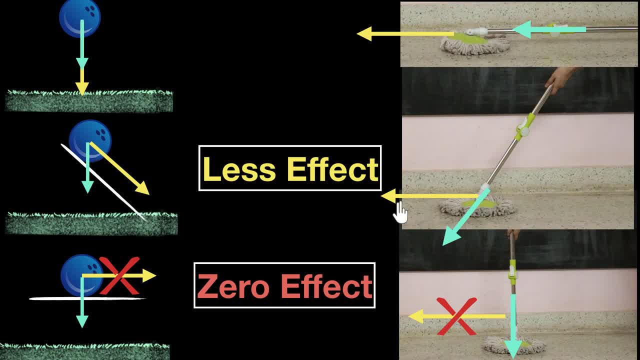 we saw that forces can have effects in other directions as well. But what's important is that forces have maximum effect in the line of the force And as the angle between the motion and the force increases, its effect starts decreasing And eventually, when the angle between the force 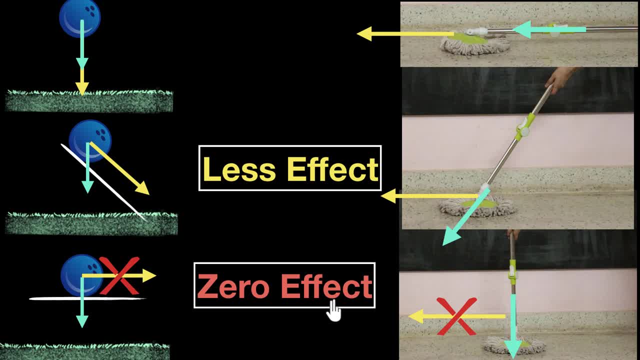 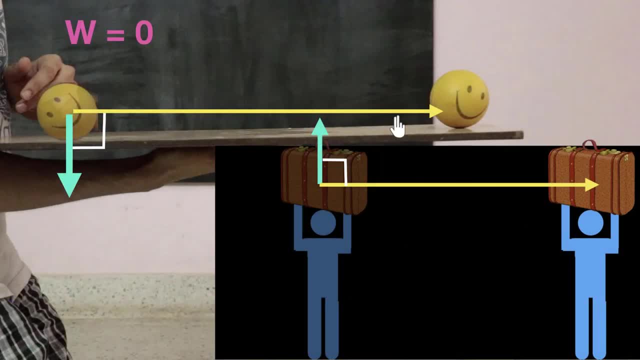 and the motion becomes 90 degrees, we see that the force has zero effect. Forces have zero effect in perpendicular direction And because of this, if the force and the displacement are perpendicular to each other, that work done by that force should be zero.